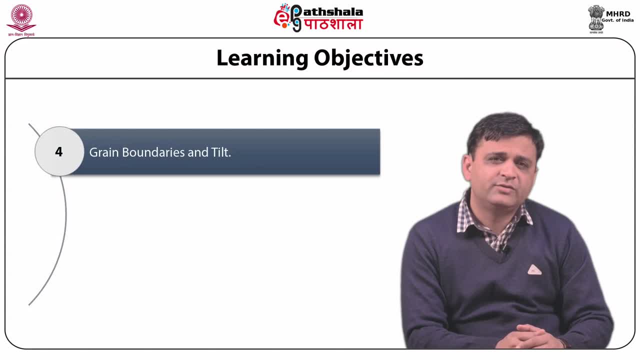 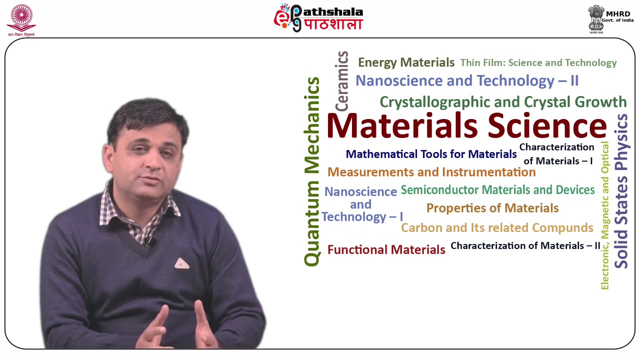 boundaries and tilting of the grain boundaries, interfaces within crystals, and also 3D defects, just like volume defects, And, most importantly, how to characterize these defects using electron microscopy. So we will tell little about these two techniques. So electron microscopy will be used for small scale, small length scale objects. And when I say characterization, 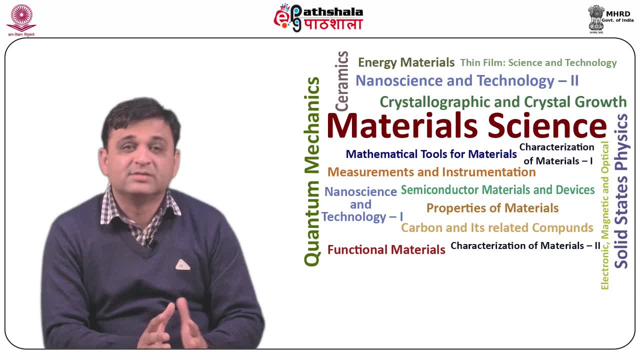 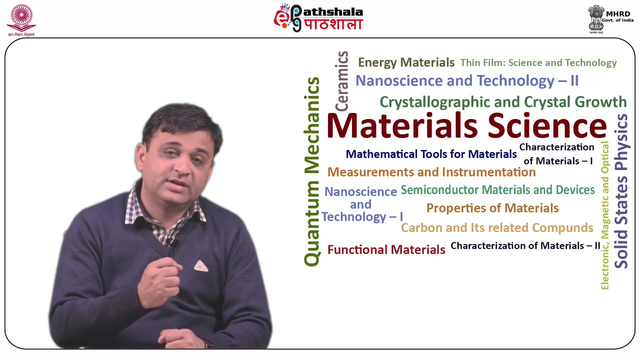 it means we want to find out types of components, 粘 out the size, the shape, all these things about the defects. now let us say what do you mean by a line defects? these line defects are so called dislocations. you have seen that if you pull material, if it, the material has a strength, it is a. 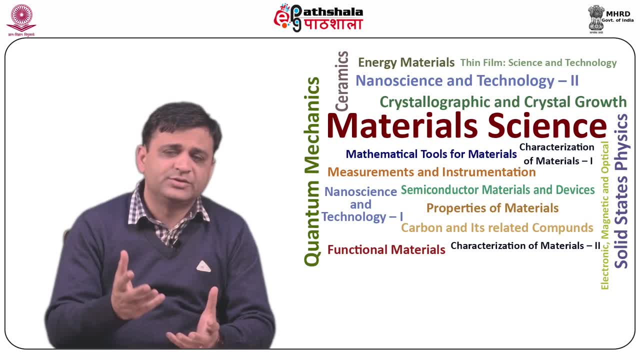 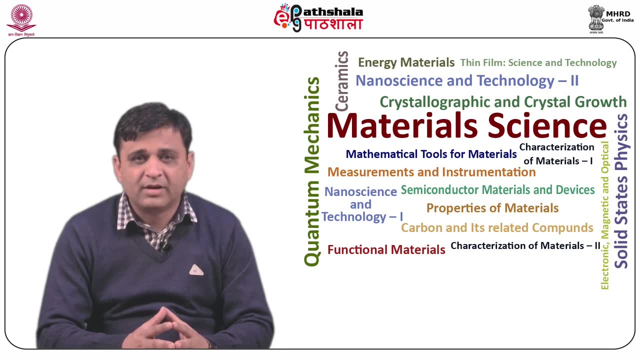 little. it is elastic. it comes back to its original shape. but when you push it or pull it beyond its limit or it causes a plastic deformation. plastic deformation is when it does not return to its original place. so usually there is a slip of the planes in this kind of deformation inside the crystal and a 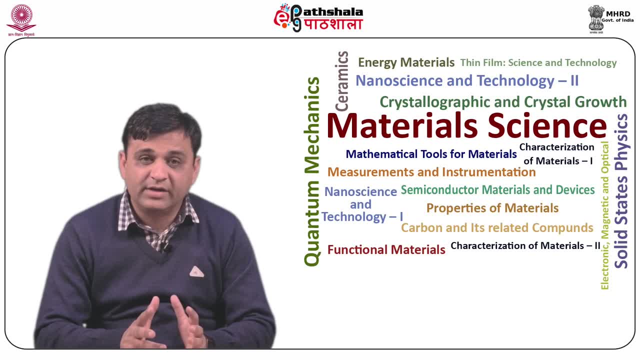 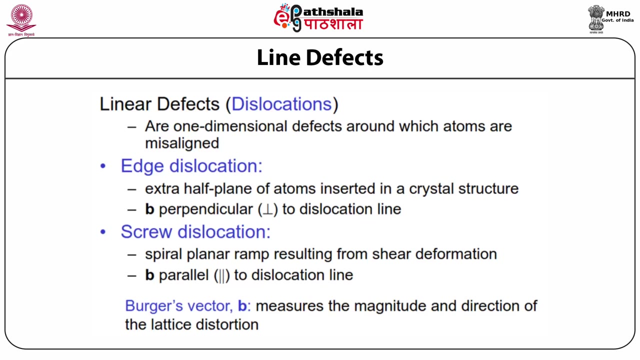 permanent deformation kind of takes place, there can be a void, or you can say the atomic bonding between some planes are disrupted completely and we have created some linear defects, some planar defects in this kind of when performing this kind of deformation to a large extent. so, as we learned, that defects can be of 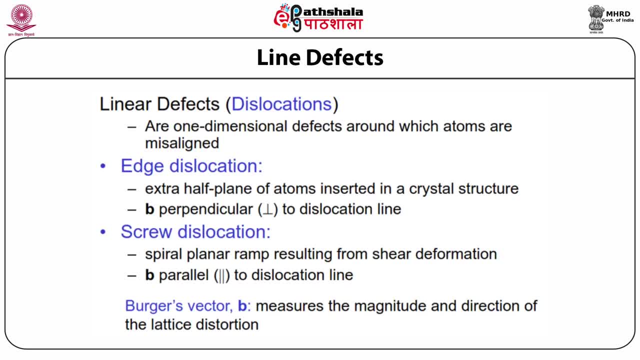 different type. we have already learned this point. defects and in point effects a lot, but we have just ONE DEDICTION, limits of defects. so we found that at some particular point, either there's an particle Board, is a missing from there, so this defect can be of different type. 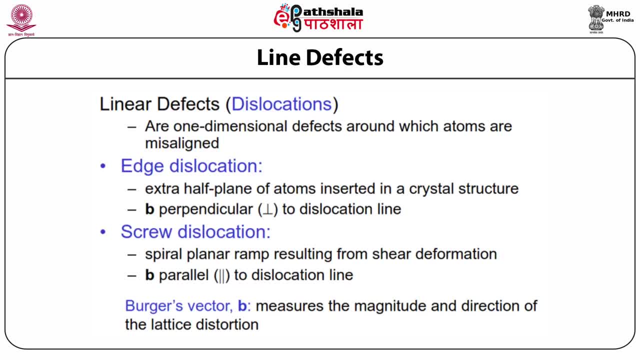 and of different geometries. so with respect to the dimensions these defects are defined. so there is another class of defects which is called line defects. so in a crystal, if you go and along a line, you find some defect, so that the defect is existing along a particular line for a sufficient distance. so then it is. 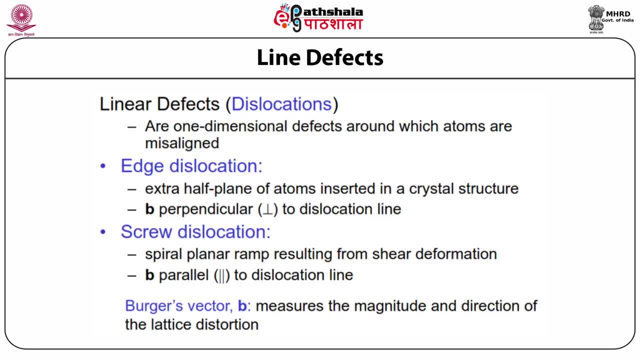 basically a line defect. so in technical language these are called dislocations. and this dislocations are one-dimensional defects around which atoms are misaligned. so in this dislocations also we have two different kind of dislocations. one is called H's dislocation and another is called 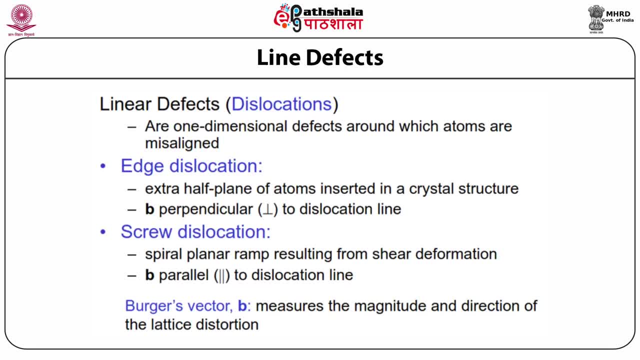 screw dislocation and of course these we will discuss in detail and in the next slides. so there is also one term called Burgers vector which will come into the next slides. so there is also one term called Burgers vector which will come into the discussion in this. so with respect to this Burgess vector, we will understand that how we 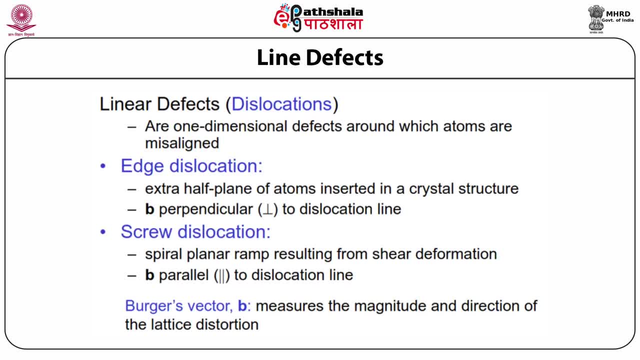 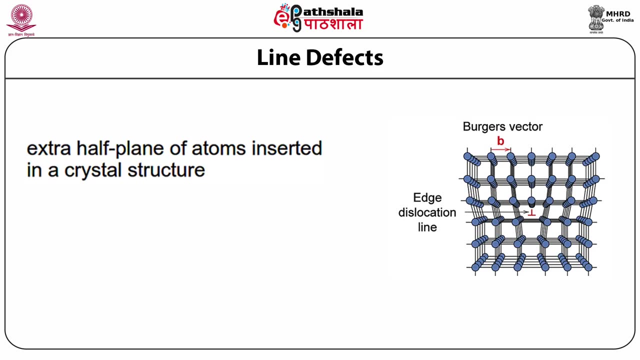 are going to classify the edge dislocation and screw dislocation and sometimes they can be mixed. also it means in a given specimen you can have edge dislocation as well as screw dislocation at the same time. so in this slide we have shown here edge dislocation. 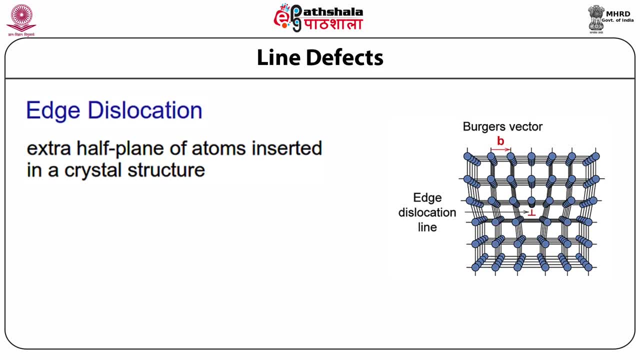 so you can see that on the right hand side we have a figure and on top of this figure- this is this: atoms or the planes are nicely arranged, but as we come below and after this third layer, there is an inverted t and below that you can see that a particular 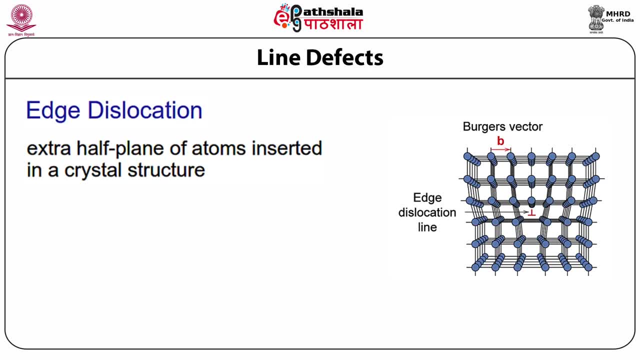 line of atom is missing just below that and due to this there is a distortion around this inverted t and now you can see that below this t there should have been an entire line so that this crystal would have been complete and there should not have been any plane missing from there. so you can see the entire row is missing. so along this line, 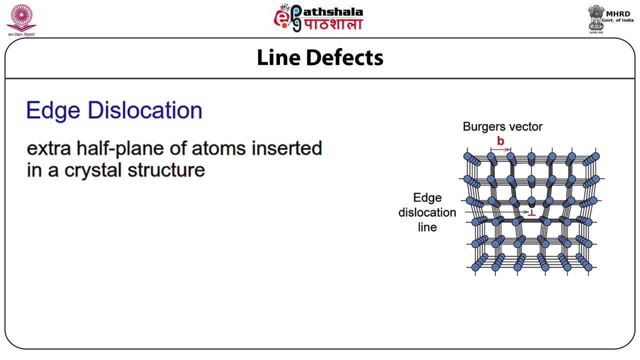 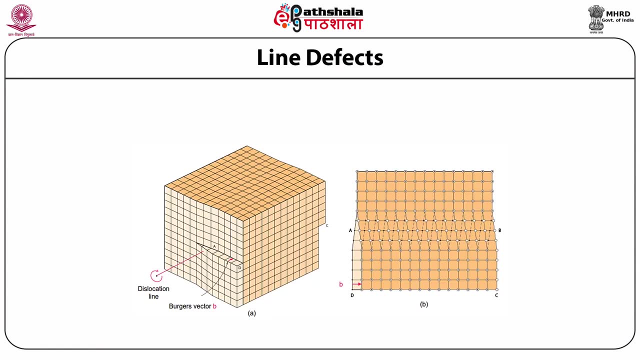 there is a defect. so that is why we call this line defect, and this kind of missing of a plane along a line is what is defined as edge dislocation. so in this slide we show you another type of line defect, that is, screw dislocation. so if we look at the diagram we can see that the geometry of this dislocation is clearly visible. 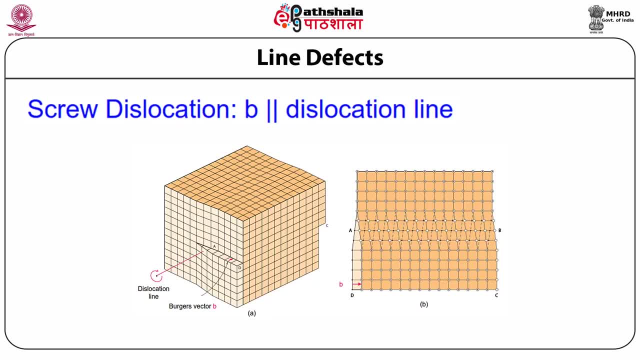 in this diagram. but let me draw an analogy: that if you have an eraser which you use for erasing when you write with pencils, so you you cut it somewhere from the middle and do not cut it through completely, but stop somewhere in between, and now you apply a twist. 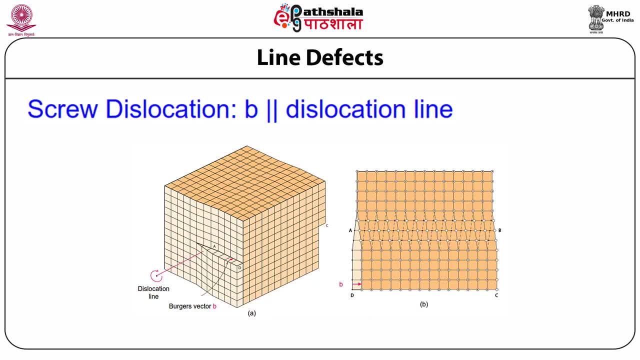 at the upper portion. you take it on the other side and lower portion on opposite side and you will see that you will find you will create a kind of shape which is visible in this figure a here. so it is as if near the point from where this cut ends. you rotate the entire entire structure above and below. 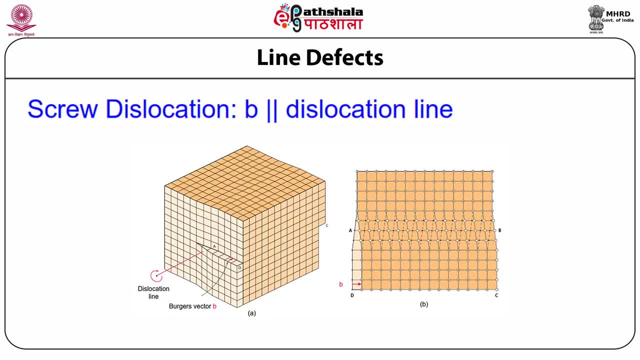 so that is why it is called as a screw dislocation. so this is: this dislocation is created due to some line perpendicular to that line. you have an axis of the rotation in this figure. now this will be more clear in terms of berger's vector, which i am going to talk in next slide. now in this slide, 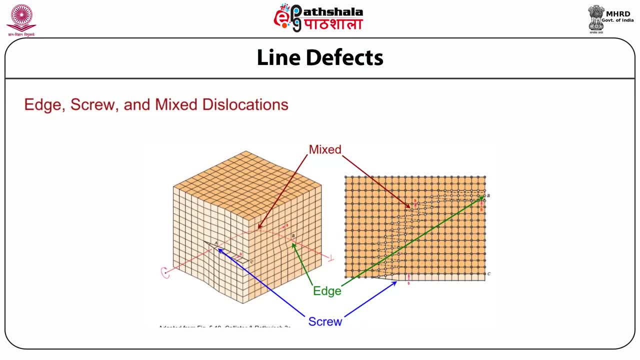 you can see that there are mixed type of dislocations. there is a blue arrow which shows a and there is a edge dislocation. they both can present at a side. so this is a mixed dislocations and when you take the intersection from the point of this dislocation. so that is. 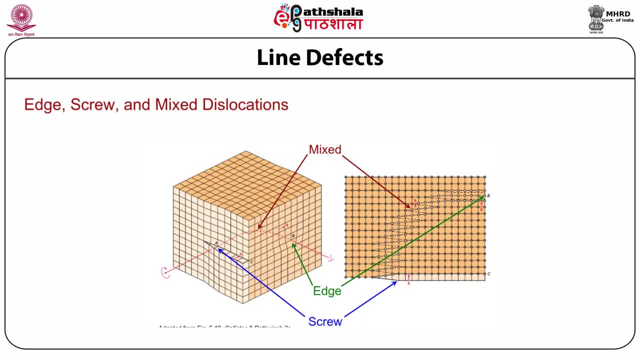 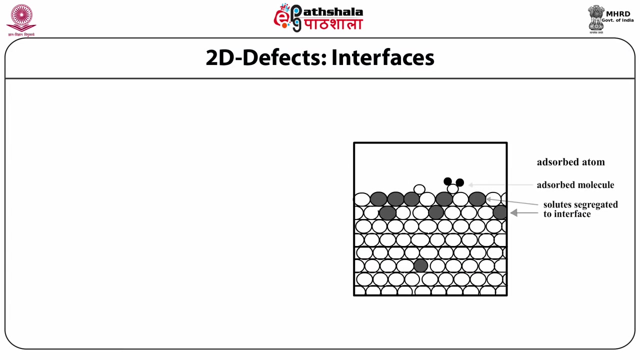 shown on the right side. that's how this dislocation. you can see that it is visible, it is. it has a particular path at which the our crystallinity or order is somewhat lost. so this is another type of defect. 2d defects: interfaces. so till now we have discussed point. 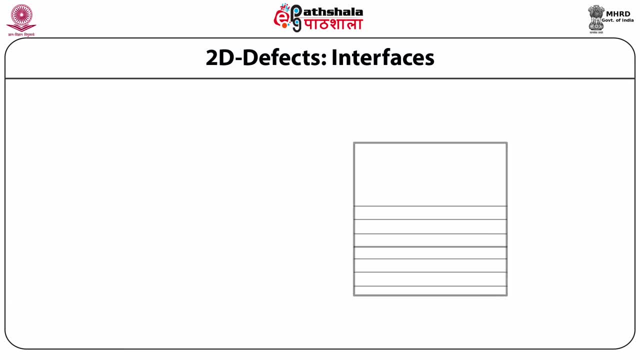 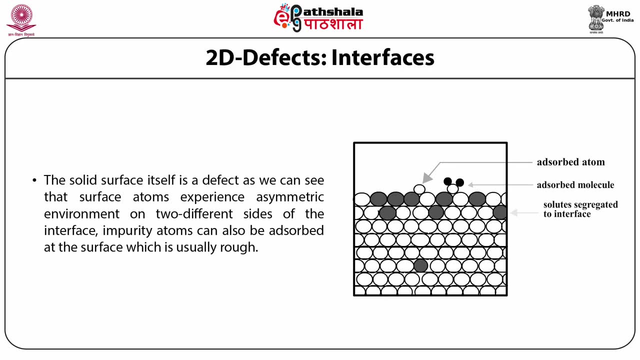 defects and line defects. now, this is a defect in a plane, so this is two-dimensional effect. so the solid surface itself is a defect, as we can see that surface atoms experience asymmetric environment and they are in the form of two different sides of the interface. impurity atoms can also be. 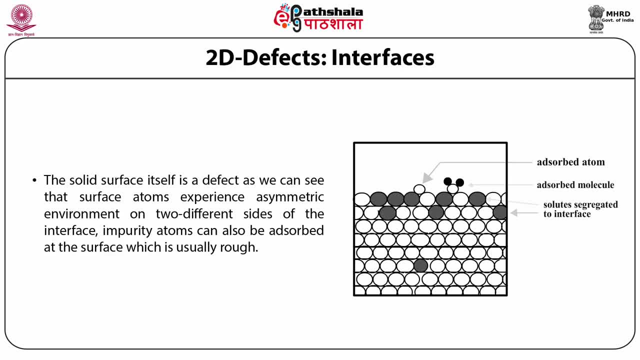 adsorbed at the surface, which is usually rough. so the idea is that when you see some atom which is buried deep inside a crystal, now it has a symmetric environment. i mean on all sides you can see that it is bonded with atoms and it is not exposed to environment. 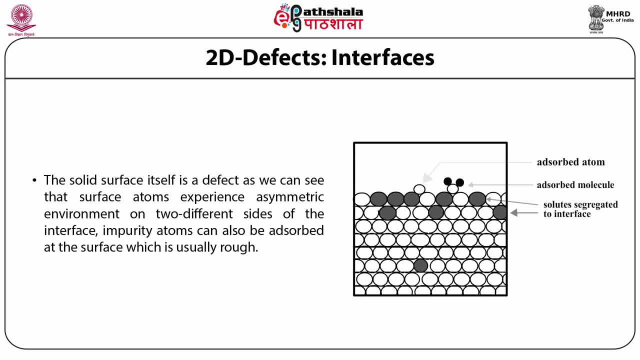 But when you come to the surface of a substance, you can see that environment is not symmetric for the atoms which are sitting on the top. On one side they are bonded with solids, on the other side they are exposed to environment. So when they are exposed to environment, some atoms, gas molecules, can interact with the 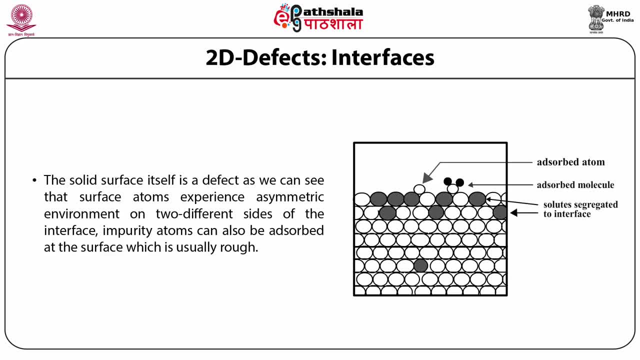 top atoms. they can chemically bind there, they can physically bind there or can also diffuse to certain extent inside the solids. So this kind of defects you usually see that they exist in a plane. So there is a plane in which this layer of or concentration of defects will be there. 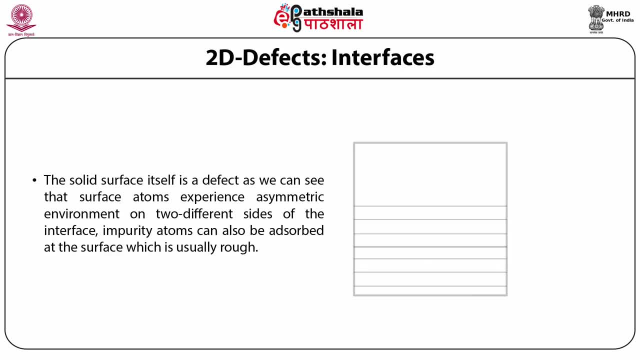 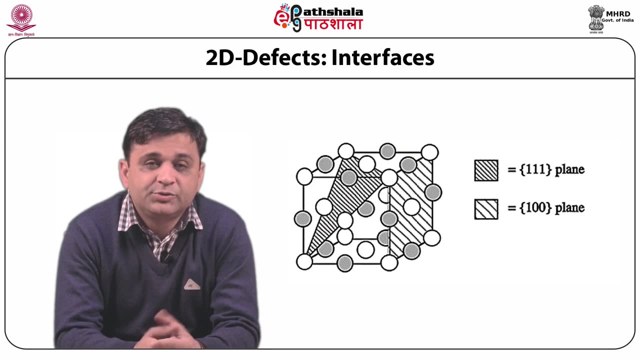 near a plane. So that is what is called two-dimensional defects, and that study of two-dimensional defects is a subject of survey Surface physics. so one can study this under the area of surface physics. So we are talking about 2D defects. 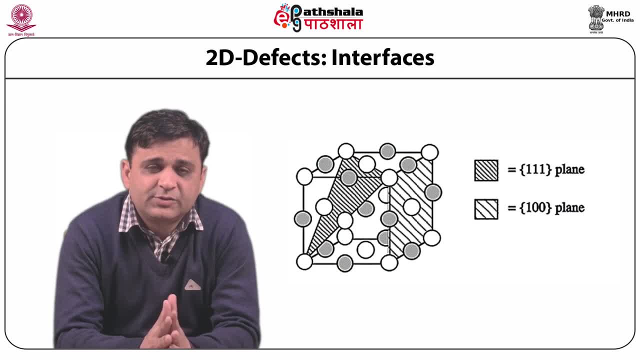 So there is also this one kind of defect due to the unbalanced electrical nature of the planes. The interfacial tension of a surface in ionic solid is strongly affected by the distribution of electric charge, As you can see in this figure. this is a figure of sodium chloride showing an electrical neutrality. 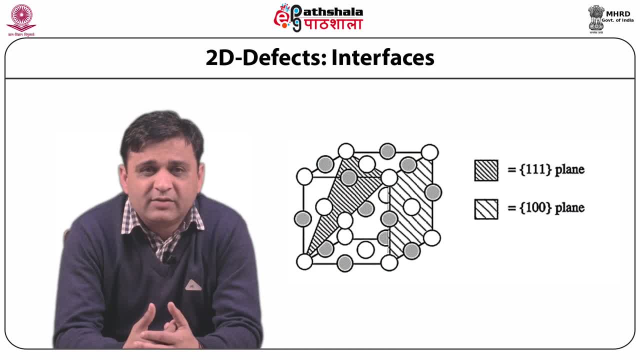 in certain planes and in another plane it is not electrically neutral. So plane is electrically neutral and plane is not electrically neutral, As you can see that on plane you have equal number of positive and negative charges. So you can see this, the surface of plane. apparently it looks to you that there. 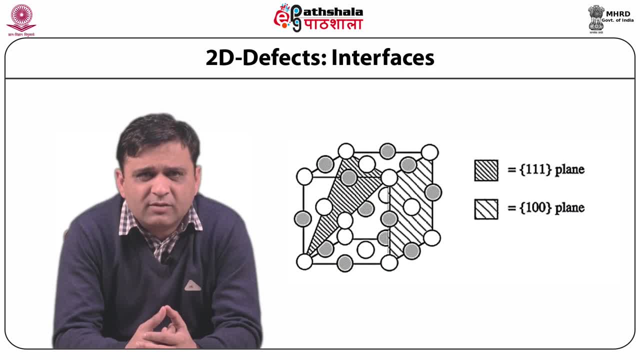 are five white balls and four dark balls. So how does it define neutrality? You need to understand that from all these four corners, one upon eighth portion is contributing. So this half atom is contributed from all four corners and half atom is contributed from the face. 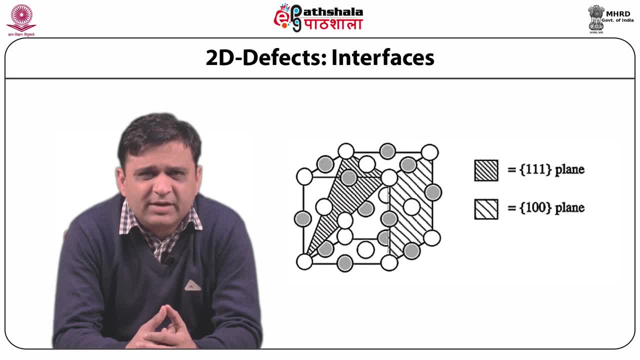 So this constitute a one atom. Similarly the four dark atom at the edges they also contribute one fourth each. So there is an equal amount of positive and negative charges. So it's electrically neutral. It does not influence another layer which is of the same family, and because this will, 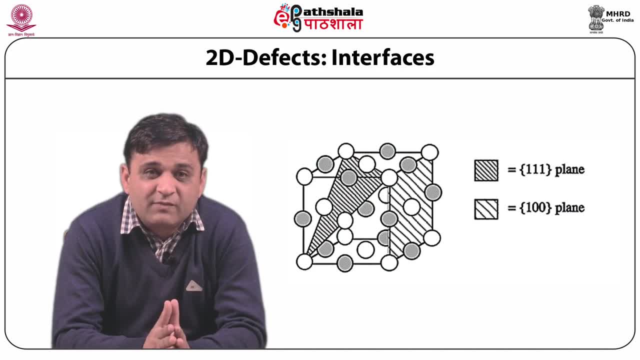 have also electrical neutrality. But if you see one one, one plane, there is an axis of a positive charge over there. So this is a positive charge over there. So this is a negative charge over there. So this is a negative charge over there. 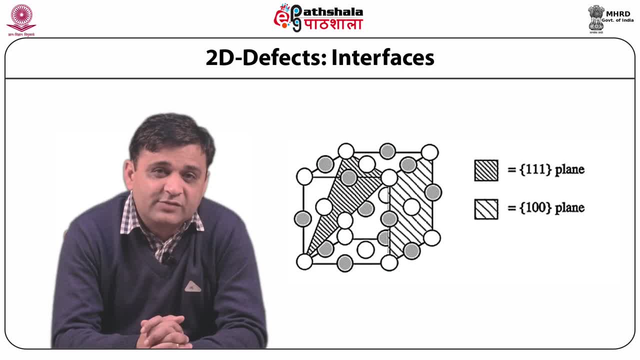 Or in another plane there will be axis of negative charge, So that creates a kind of electrostatic interactions between these planes And so that is you can say that cause a defect in the plane. It could lead to local distortion in the system. 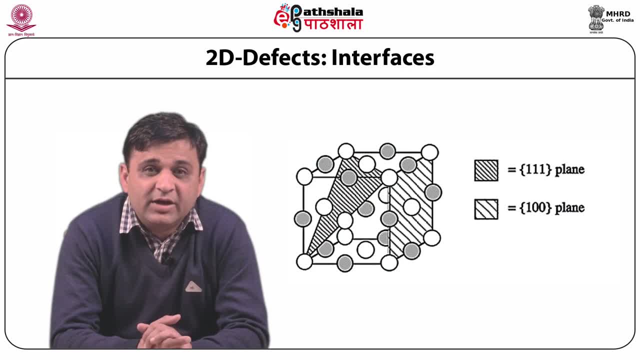 In strong ionic materials, the electrically neutral surfaces- one zero, zero- have all the same characteristics. So this is a negative charge over there. So that is a positive charge��� over there. In lower, classify you. You see a change. 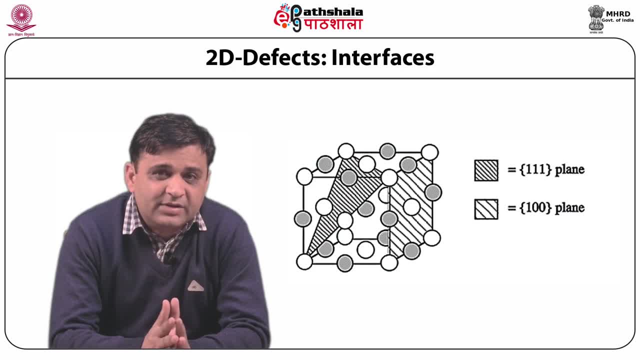 This is some fude in the material Over there. it's in two. One is nuclear. That's the fude. There's purpose in that and some some sort of work with the surfactant materials which are itself charged, and when we apply these materials to such kind of surfaces we can neutralize it. so basically, 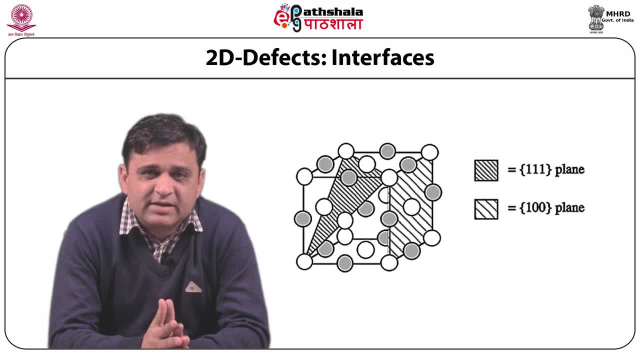 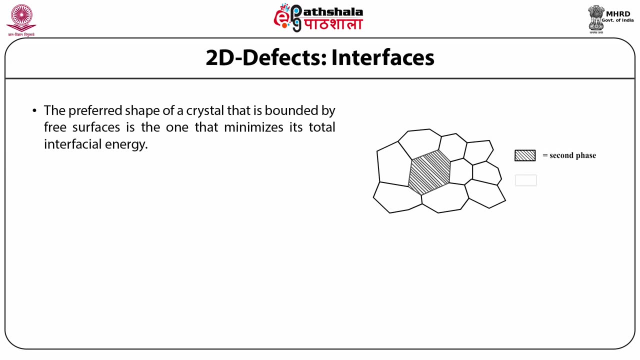 we can fabricate or synthesize some different kind of charge environment. given this kind of charged planes interfaces between crystals, the preferred shape of a crystal is bound by free surfaces- is the one that minimizes its total interfacial energy. the macroscopic surface of the crystal can always be treated as if it were made up of facets, the kth, one of which has an area. 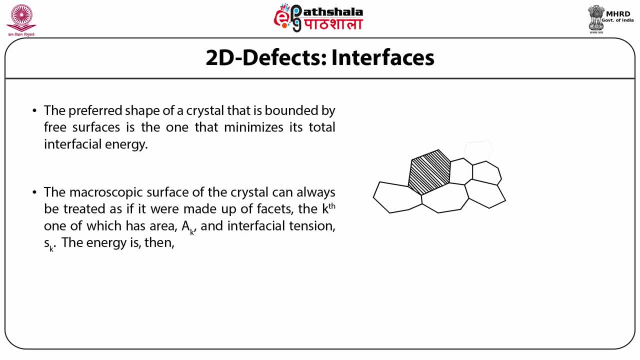 ak and interfacial energy. sigma k: the energy is there. e is equal to sum over k. sigma k: ak, which is written in the formula. so you can see the diagram on the slide on top, which which is an entire solid and it is basically a collection. 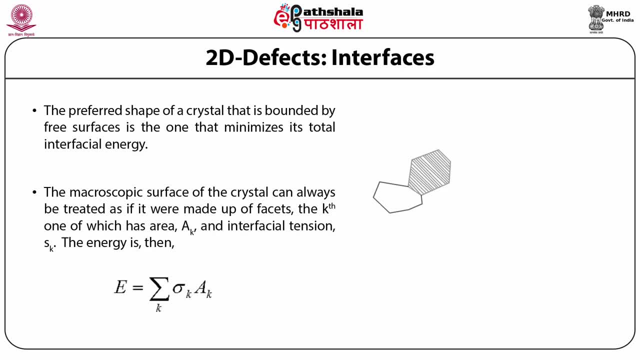 of pieces. you can see that because this is a three-dimensional system and on just because we are drawing it on the slide, we cannot see all three dimensions. but you can see that each of the the portion of this is attached to nearby portion and there is a boundary in between. 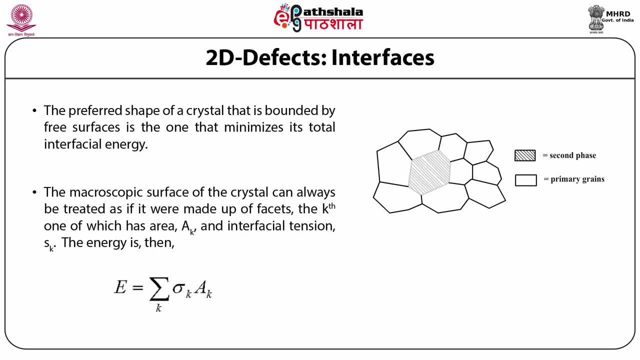 the grain. so these are crystalline grains and this is usually the samples or crystalline substance we get in laboratory, where their nature is polycrystalline- entire system is hardly single crystal. or if it is not made so, then we call it polycrystalline. but this is not polycrystalline. if you do not have a polycrystalline, 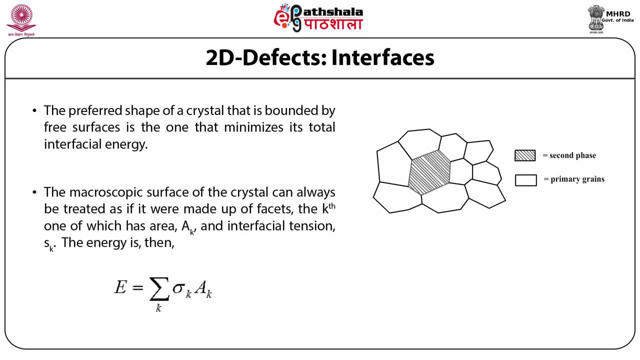 material, then you can make your own with the some special purple. usually you get polycrystalline materials, so you can understand that when you cross a boundary between one grain to another grain there is a symmetry breaking in terms of translation and in between the boundary, some of 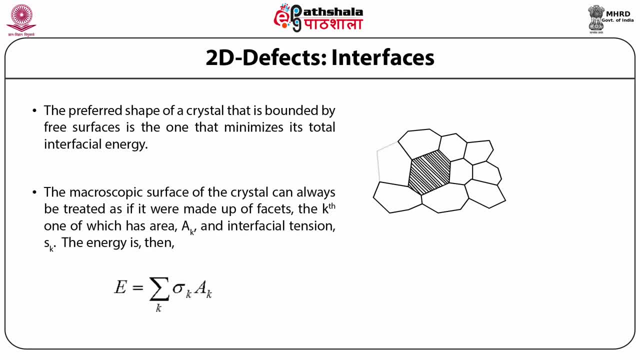 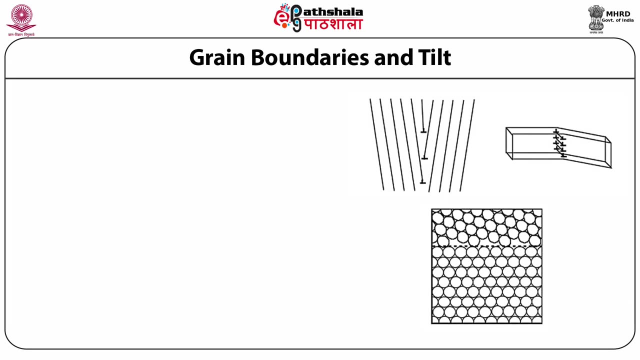 the area is disordered and that disorderness goes along a plane. so this is another kind of is attached to another facet, so this is called interfacial defects and those exists in polycrystalline samples, grain boundaries and tilt. a tilt is a vertical. 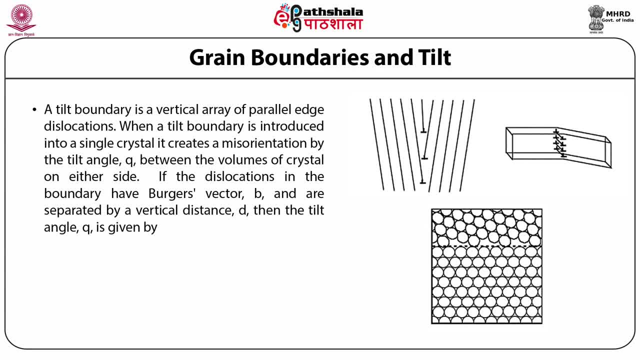 array of parallel edge dislocations. when a tilt boundary is introduced into a single crystal, it creates misorientation by a tilt angle, theta, between the volumes of crystal on either side. if the dislocations in the boundary have Burgers vector B and are separated by a vertical distance D, then the tilt angle. 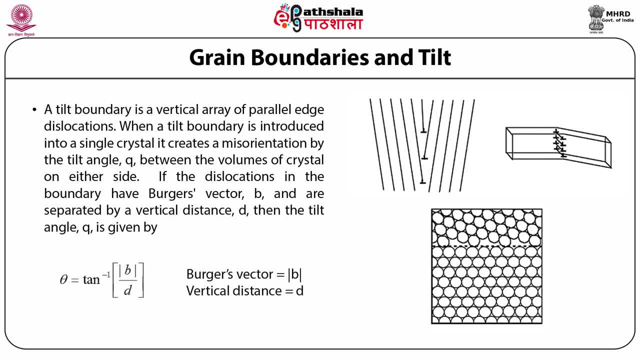 theta is given by the formula: theta is equal to tan inverse B upon D. so as you can see the same in the left hand side in the figure that there are two kinds of grains with the parallel lines, these are the crystalline planes and they are with each other and there is an inverted kind of T. So these are dislocation lines, perpendicular. 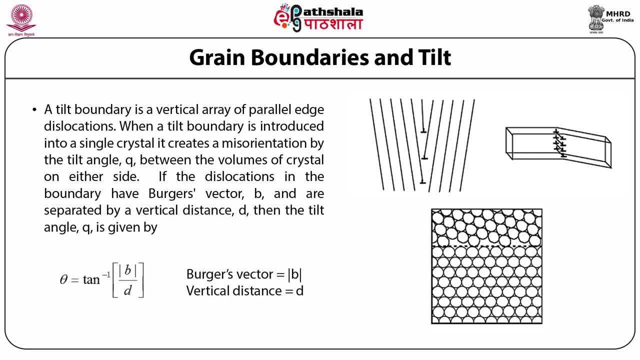 to the plane and the separation between these T is D in the formula. So idea is that we can determine this tilt between the plane boundaries using diffraction method. We can also use direct microscopic methods and electron microscopy and we can then calculate Burgers. 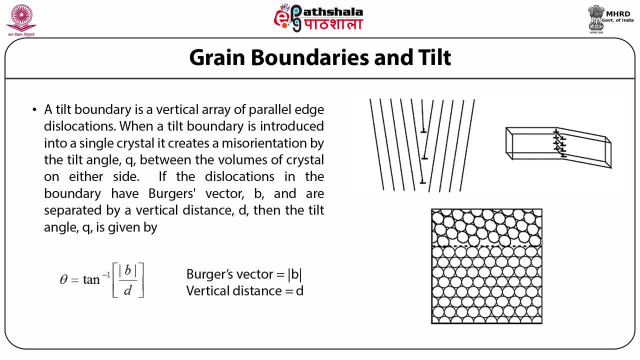 vector. using this given formula, or if we know the Burgers vector, we can calculate theta. So on the left hand side, bottom, you see a figure. there is a dotted line in between two phase. So this dotted line shows that there is a plane and this plane is perpendicular to this board. 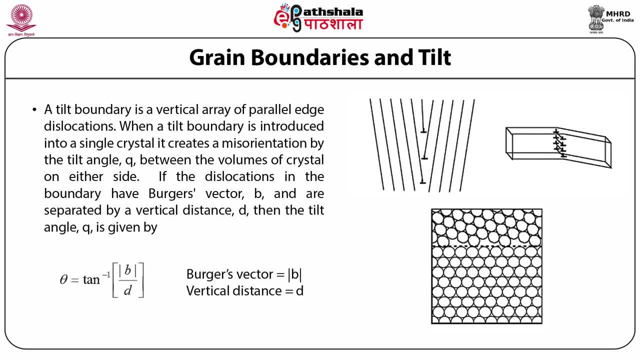 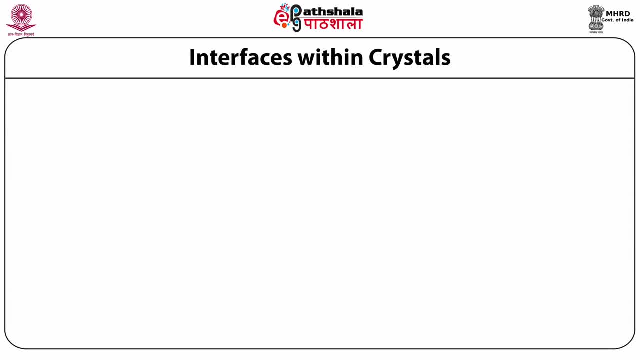 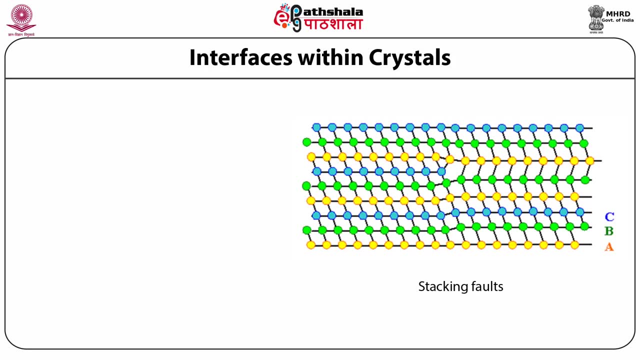 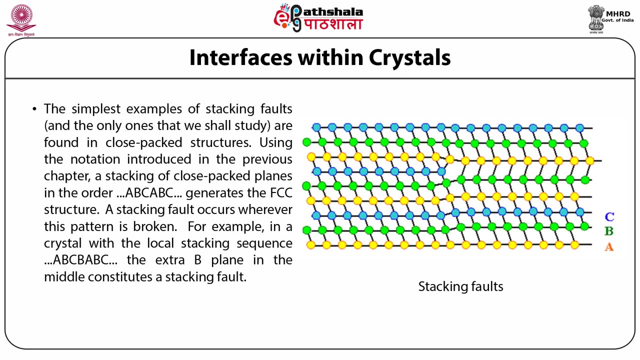 And screen. So this is one kind of plane dislocation. we know Interfaces within crystals, or stacking faults. You can see there is another type of defects which can occur in crystal. The simplest example of stacking faults are found in closed pack structures. using the notation 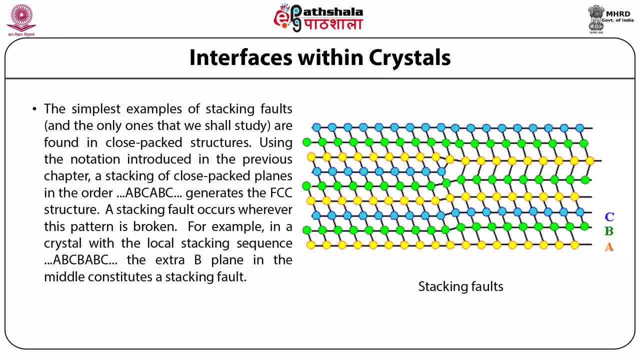 introduced in the previous chapter. A stacking of closed packed plane in the order ABC. ABC generates the axis structure. A stacking fault occurs whenever this pattern is broken. For example in a crystal with the local stacking sequence ABC, BA, BC. the extra B plane in the middle constitutes a stacking fault. This can be extra B plane or there. 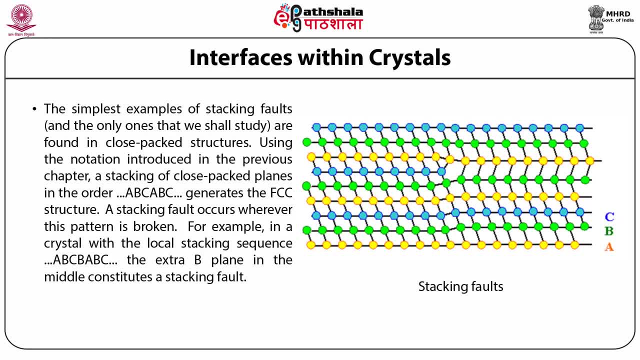 be a missing plane and, as you can see that in the diagram it is shown in three different colors: ABC, and then a, B and you can see that the C type. there is some extra point, some extra line has been introduced on on left side, left hand side, so this has created a kind of a stacking fault with respect to on the 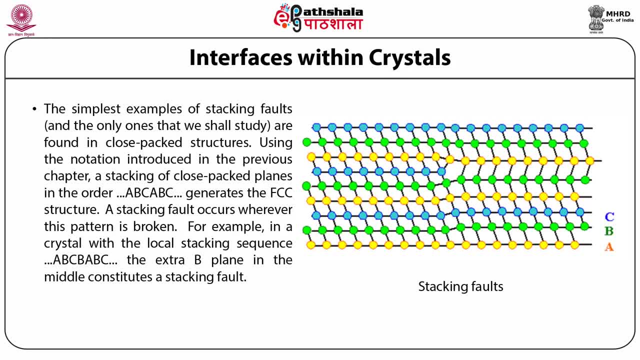 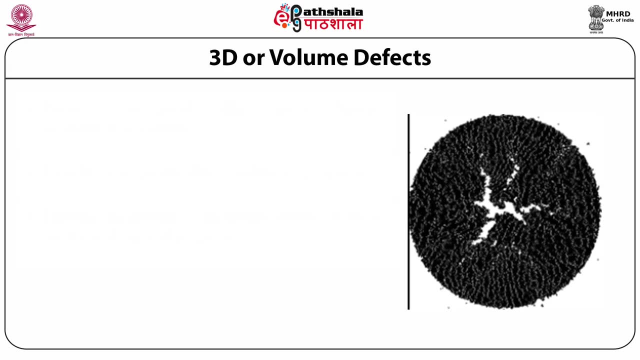 other side. so you can see that we have here dots which are repeating one after the another and on the other side that repetition is missing because of this stacking fault, 3d or volume defects. so let us also mention this: 3d and volume defects. so these are pores, cracks and foreign inclusions. so pore can greatly. 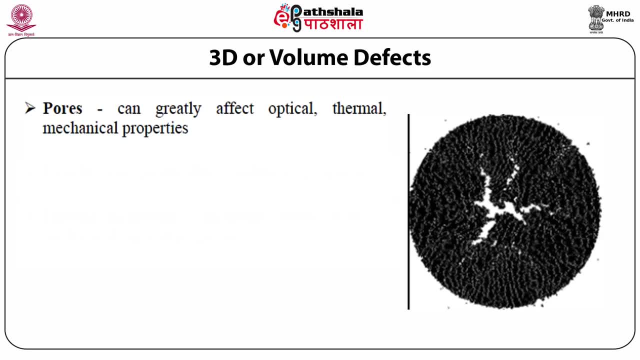 affect optical, thermal, mechanical properties. so pore is basically: it's not missing of one or two atoms, it's, let's say, some large number of atoms are missing from some place. so that creates a void. so it's a three-dimensional defect, it is. it is different from point. 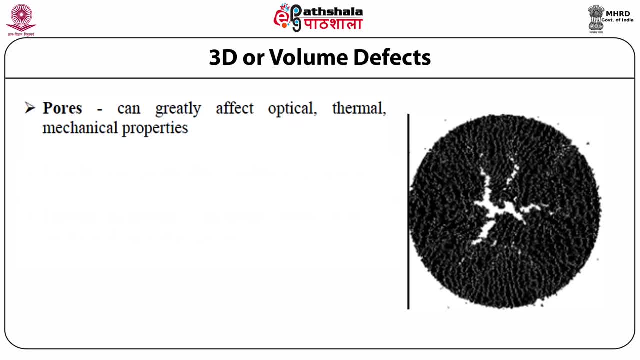 defect in point effect. maybe one or two atoms are missing and then cracks and as you can see in the diagram. so that is a is a three-dimensional defect, because it goes along all three dimensions and so we can have some foreign inclusions. foreign inclusions means some extra. 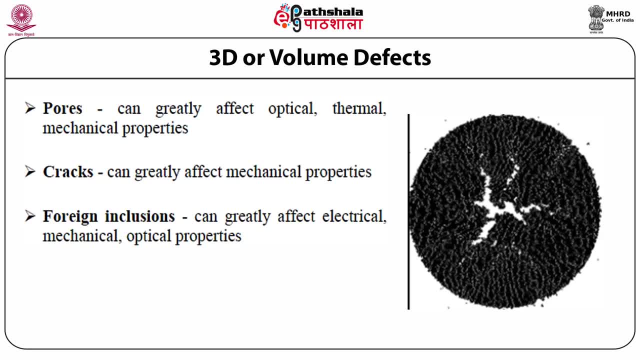 material in in the pore or cracks is filled from somewhere at a length scale quite large. so that also is a sort of three-dimensional defects in the system and this affects the property of the material and at large length scale. this occurs at the large length scale, so it will have its own consequences. so 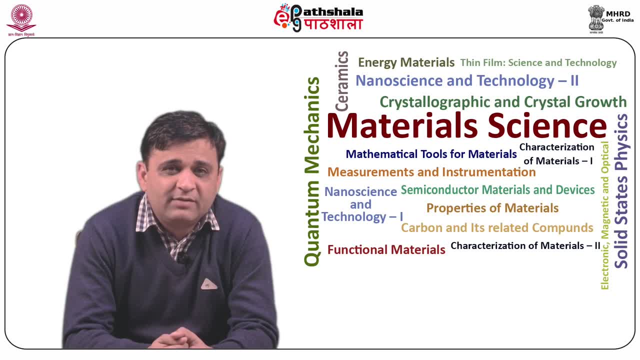 what we have learned in this module. so we have learned line defects. there are two kinds of line defects. one is edge dislocation and another is a screw dislocation, and we can identify them with respect to the Burgess vector. and another type of defects are surfaces and interfaces of crystalline material act as a as a 2d defects. so surface itself is a defect. 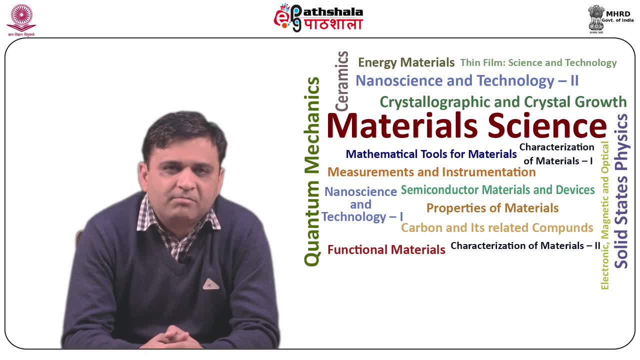 interface itself is a defect and foreign atoms adsorb at the surfaces leads to additional defects if you have a surface and you have some chemical adsorption or physical adsorption of this atoms on the surface, so that is another kind of defect, since the materials are usually polycarbonate. 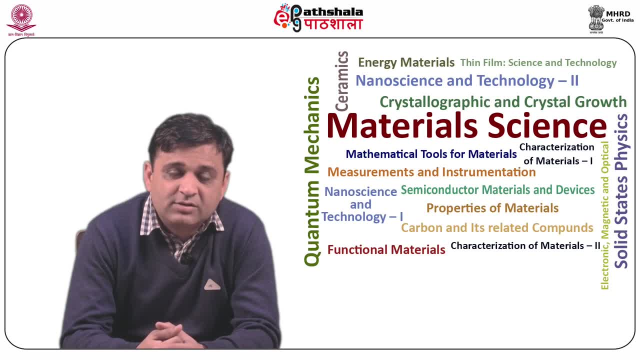 but when we cross between the two kinds of defects, the boundary of the crystal is damaged. we have a question of the boundary of the crystal is damaged. so I think one of the points that we should be interested in is that this is a surface that is acting two parts at the 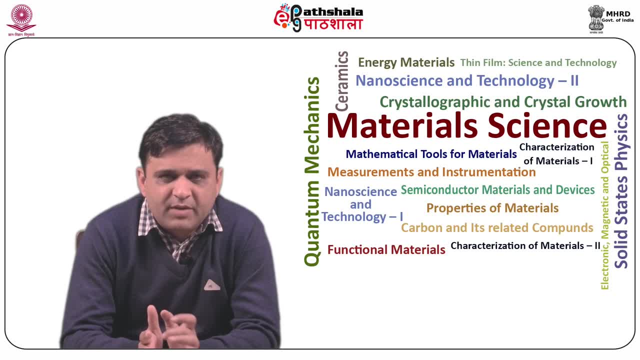 same time- and we can give some example of that- and if we give the surface location to the other one, that this is a surface, it is not working in that way because of one of the defects, and so we have another two points that could be explained here. I have some examples. 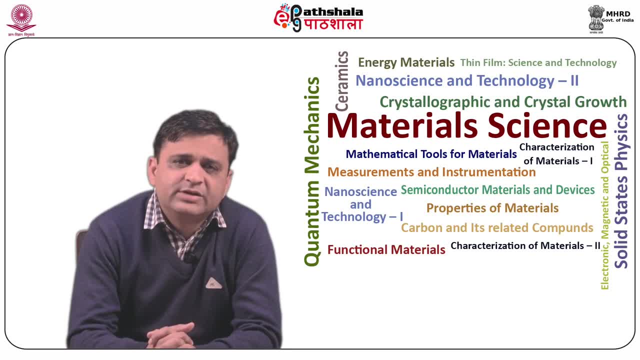 so I will explain them in a minute. I don't want to spend a lot of time here. but you is a two-dimensional defect. grain boundaries are two-dimensional effects. and then we also learned about a stacking faults, that when you are having a certain type of plane, let us say a, and you have. 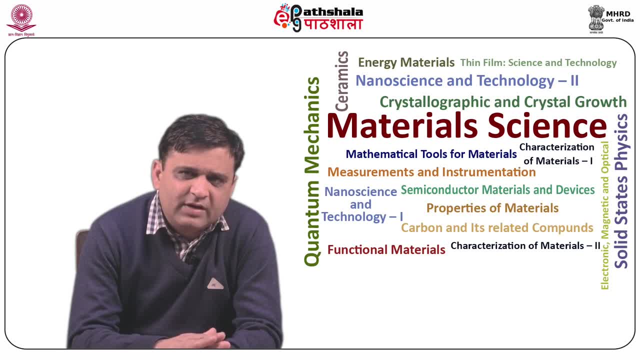 another type of plane. let us say b and then you have c. so there is a stacking of a, b, c, like this. if it goes like that, sometimes this stacking, there can be problem in the stacking. some of the order is missing. let us say complete c is missing or complete b is missing.